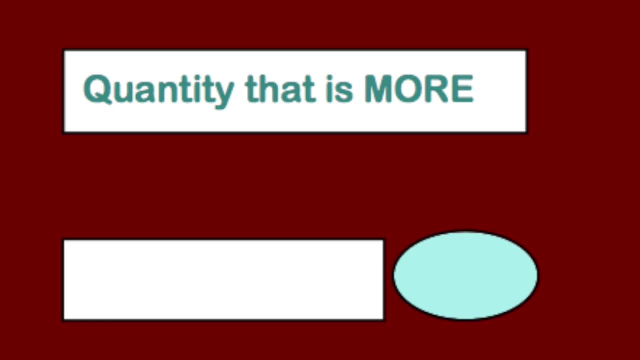 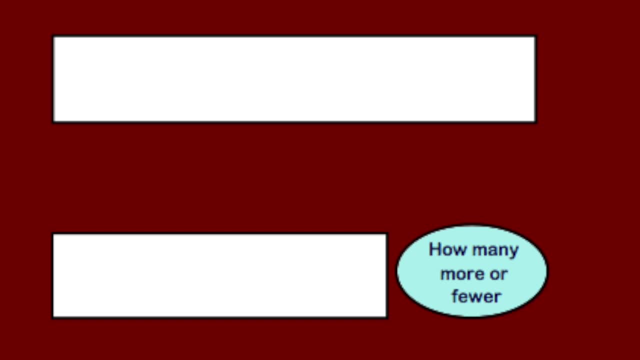 each of the rectangles and the oval: Who has more goes on top, who has less goes on the bottom rectangle and how many more or fewer goes in the oval. In this video, we will be looking at how to find the unknown number. To find the unknown number. 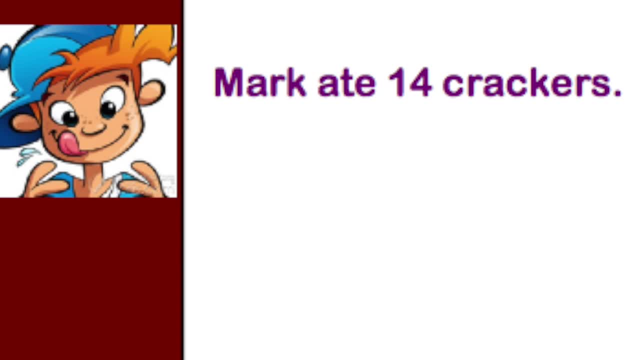 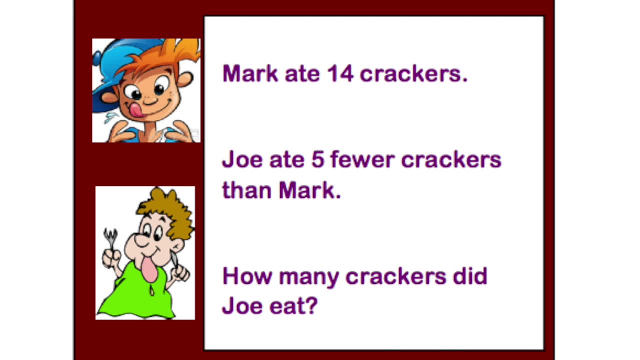 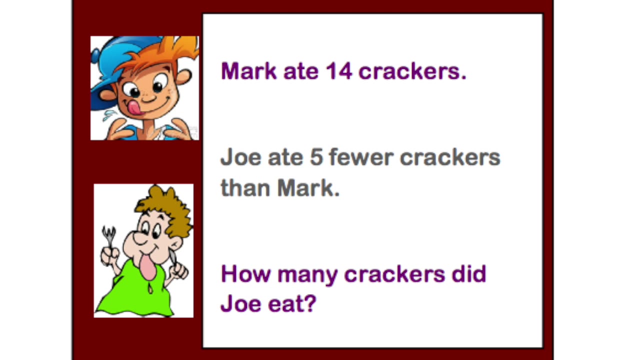 we will need to find the unknown number. In the example. Mark ate 14 crackers. Joe ate 5 fewer crackers than Mark. How many crackers did Joe eat? I am comparing how many crackers Mark and Joe ate. First I need to determine who ate more crackers. In the second sentence it says Joe ate 5 fewer. 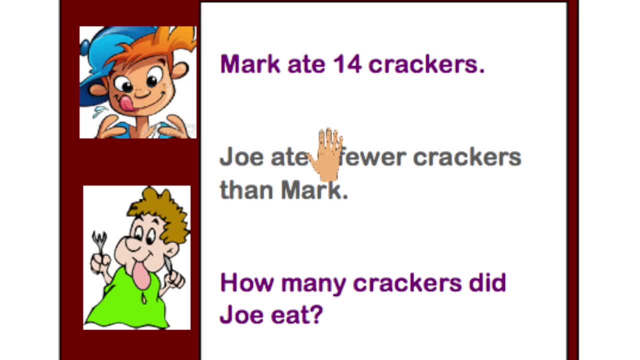 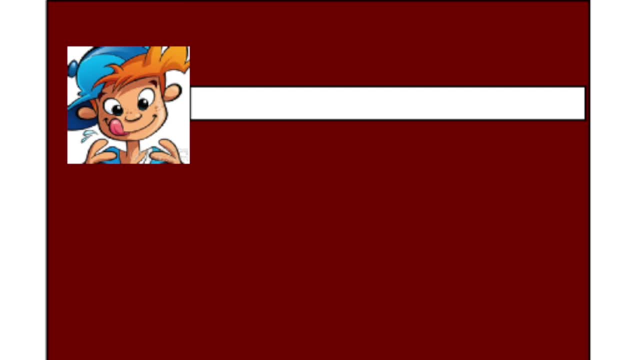 crackers than Mark. If I cover up the 5 and read the sentence Joe ate fewer crackers than Mark, I can determine from that sentence that Joe ate fewer than Mark, which means the amount of crackers that Joe ate will go in the smaller rectangle and since Mark ate more, his amount will. 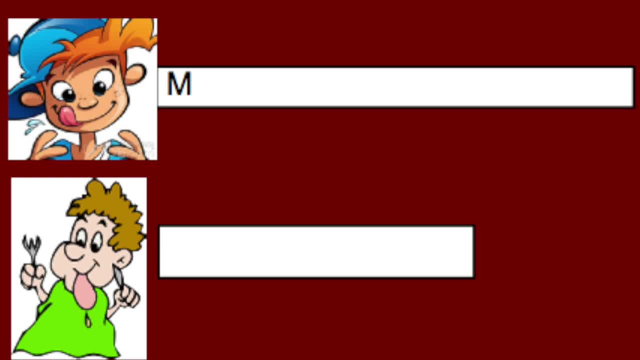 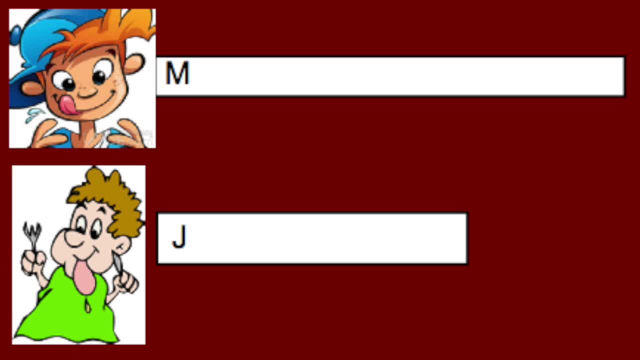 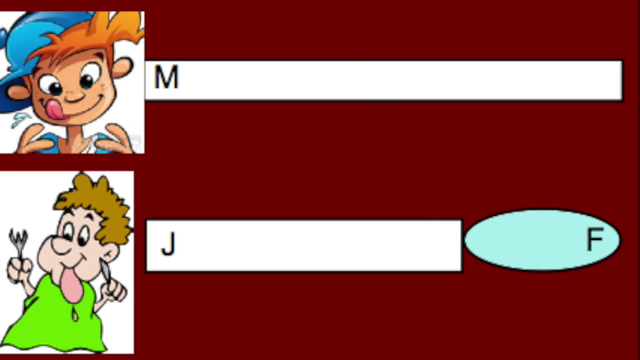 go in the larger top rectangle. I can label the top rectangle with an M and the bottom rectangle with a J. The oval can be labeled with an F to stand for how many fewer. Once students get the correct labels on the comparison bars, they can begin to put the numbers. 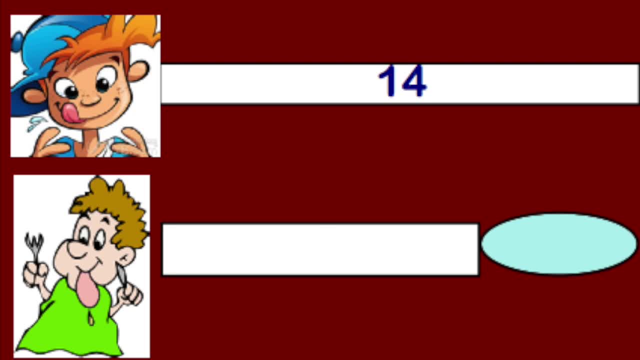 into the correct spots. So 14 would be on top in Mark's box, a question mark would be in Joe's box and the rest will be on top of the other boxes. on Mark's box It is important to remember that if you use the correct jot you are missing out on the correct number. 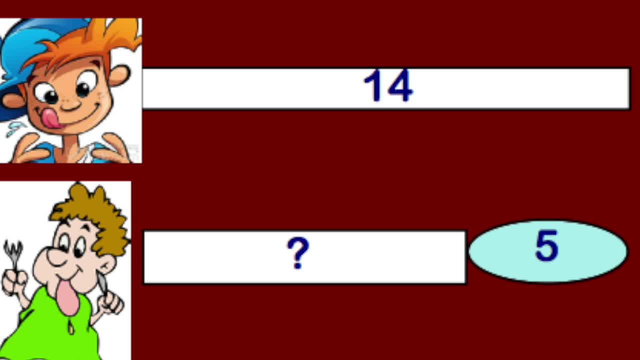 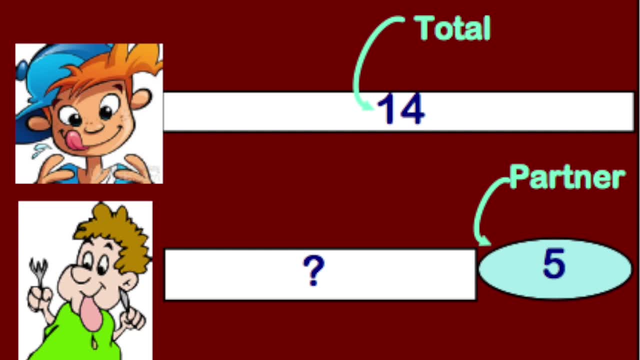 If you would like to change the number with the correct number, you will also need to select the correct number, and the number five would be in the oval. Students will be able to visually see which numbers they know- the total and one partner- and they are solving to find. 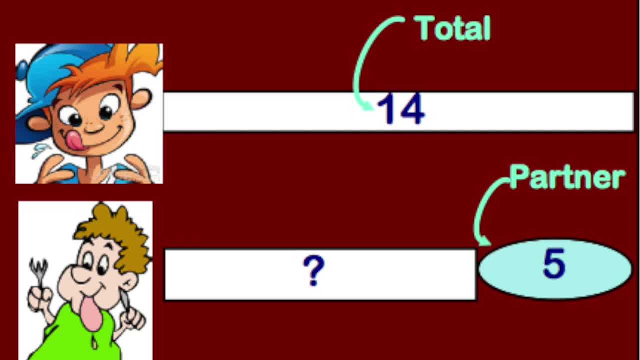 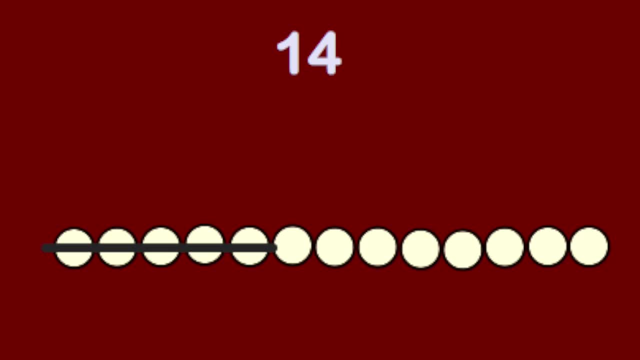 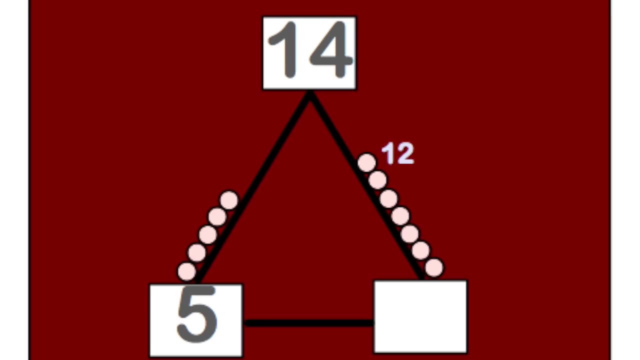 out the other partner. They can use one of the strategies they know to find the missing number. Ultimately, I could use a circle drawing and draw 14 circles and subtract five of them. I could use a math mountain and use the counting on strategy. 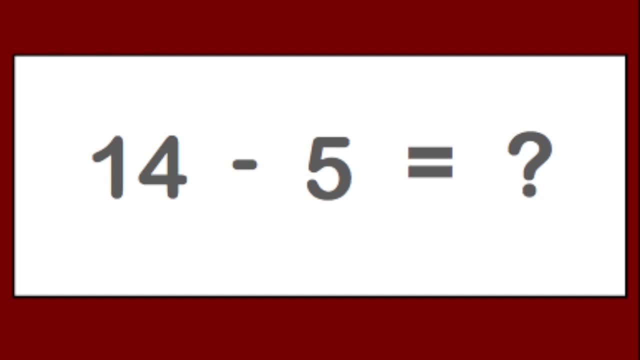 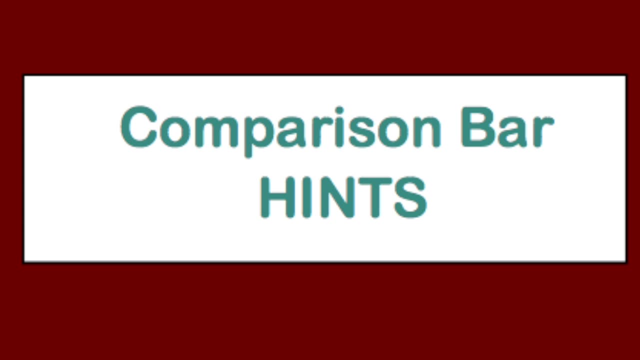 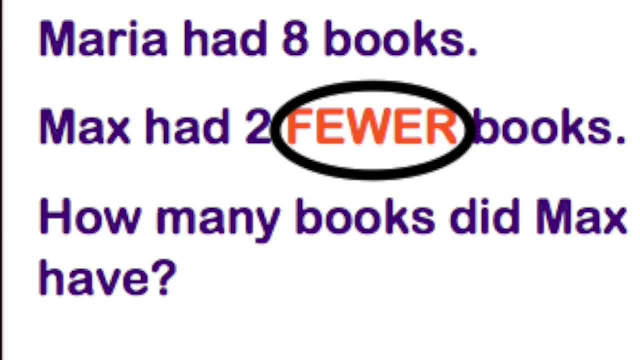 Students can make an equation if they are automatic with their math facts and fill in the missing number. Just a few hints to help get your comparison bar set up correctly. The numeral next to the word fewer or more is usually the number that goes into the oval. If you cover up the numeral that is next to the. 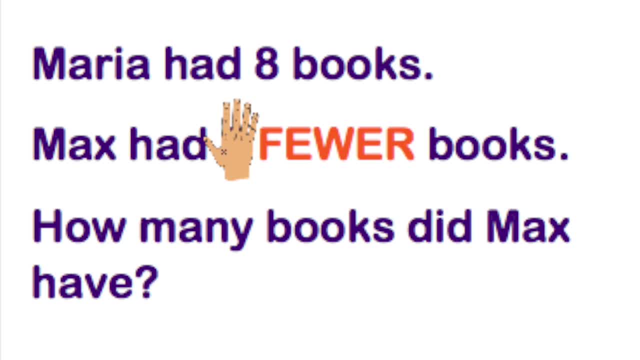 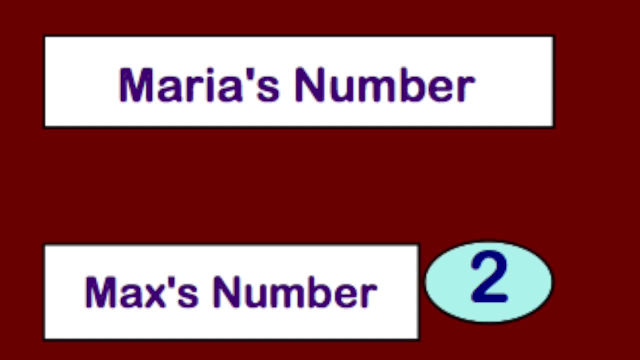 word fewer or more and read the sentence. the sentence will tell you who has more and who has fewer, therefore helping you to figure out which number goes into the larger number. Please note: in third grade the smaller quantity goes on the top with the oval and.